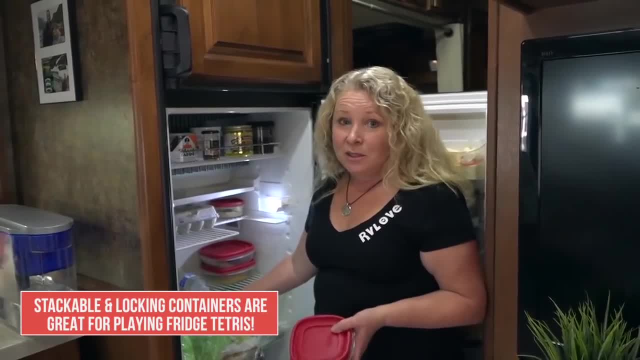 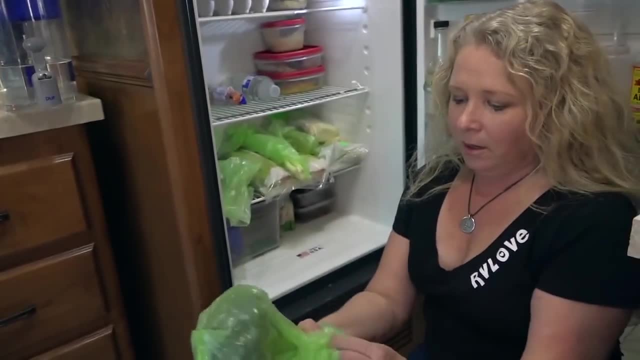 If you're really clever about it, it's a bit. it's a bit like playing Tetris in your fridge. Definitely time for a grocery shop around here. but here's what I mean about the Debbie Meyer space bags. I just use them with an elastic band and 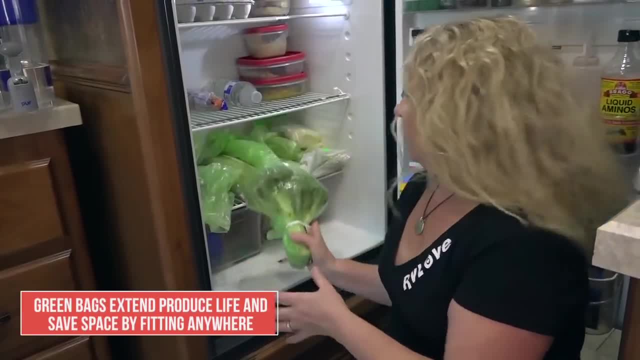 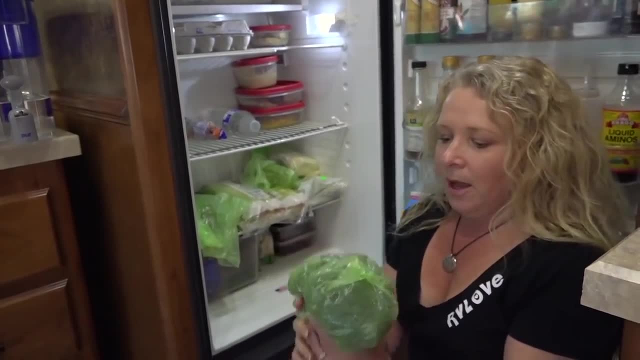 you can literally, you know- just put things in wherever they will fit. Things like scallions can pretty much fit in anywhere. When you've come back from a big grocery shop, that's really handy to be able to put something like this in that is only the size of the vegetable, instead of a container, which is a lot. 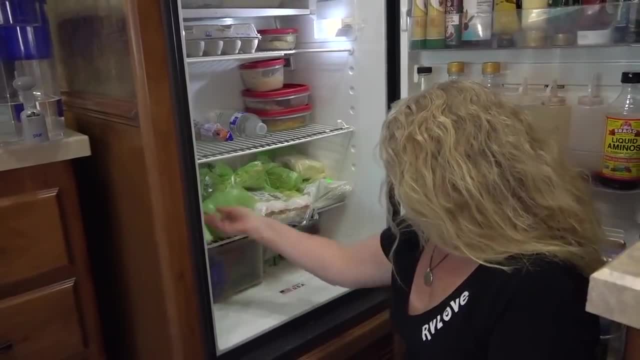 harder to maneuver But definitely need a lot of space. Definitely need a lot of space. I mean, I have a bit of a grocery shop around here. We usually have two of these. we still have the other one. We just find it more practical to keep that space open. 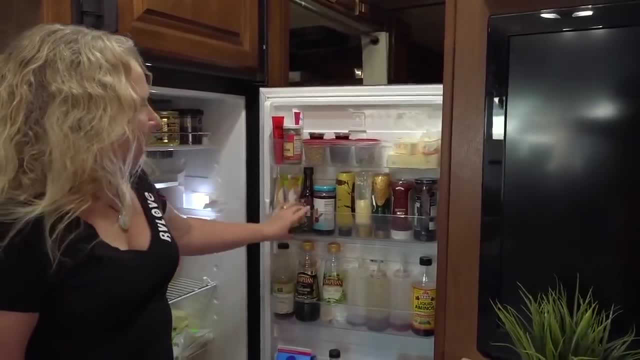 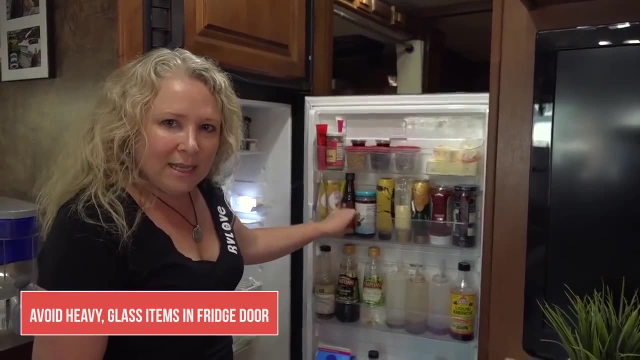 Over here in the fridge door. we try not to keep things that are too heavy here, because these are only plastic shelves, They're expensive and they brake easily. We've broken one only. I think it was cracked when we already bought the Rv. but 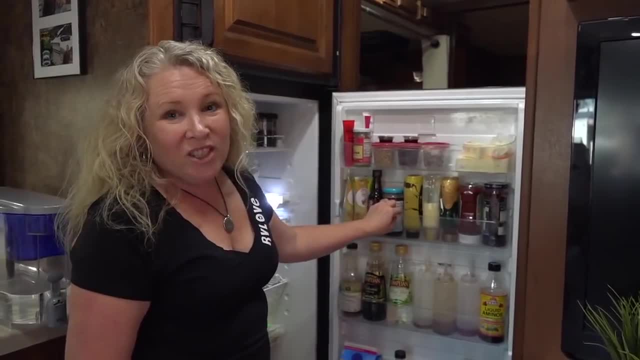 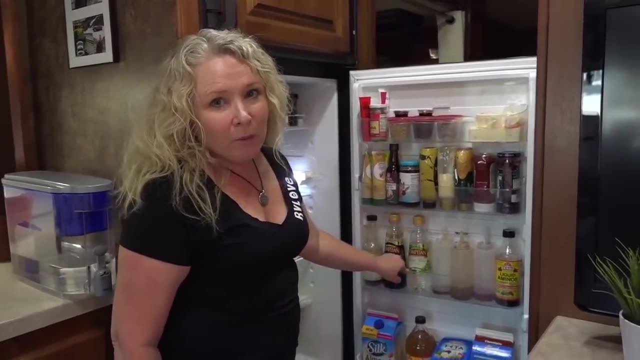 when it did break I was really surprised that a replacement with shipping cost me the best part of sixty dollars. One of these cheap crappy plastic bags for the crappy plastic shelves. So I take good care of them now because I don't want to keep forking. 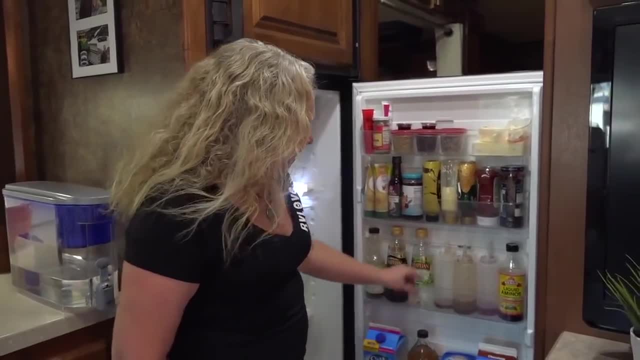 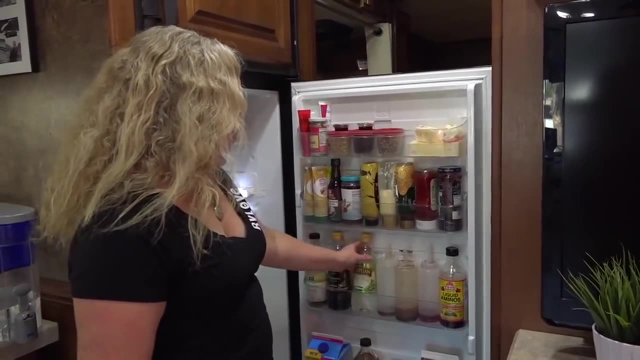 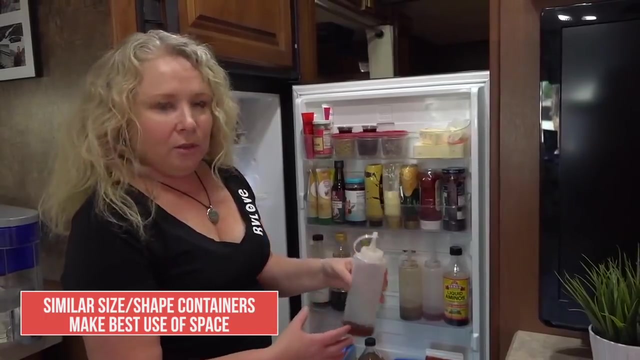 out $60 for cheap, crappy plastic fridge shelves. So these are all plastic containers, Believe it or not. these are even plastic vinegar containers, and these tend to be vinegars and sauces, And by having all the same size and shape containers, it actually is a more efficient. 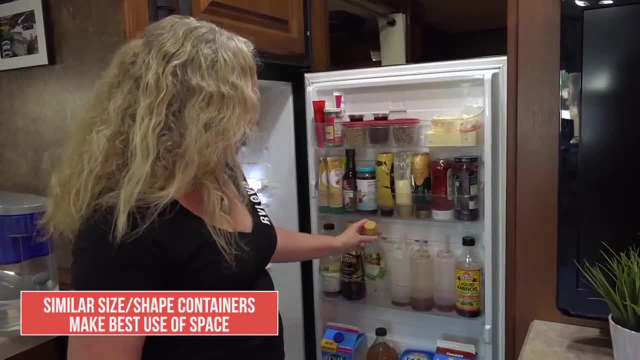 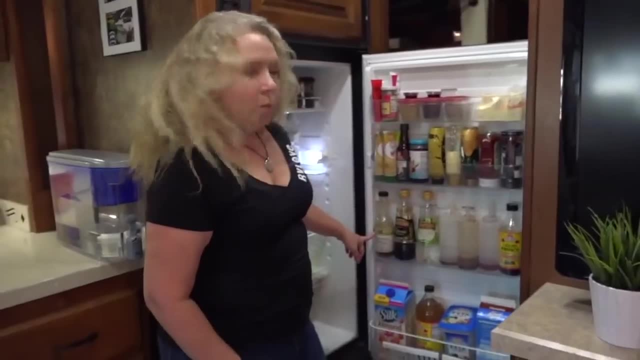 way to store them because it's maximizing. you know these odd shapes a little more limiting, but those ones aren't too bad. But yeah, you can get a lot in here with the same size and shape. but recommend plastic, obviously, ideally BPA free plastic, if you. 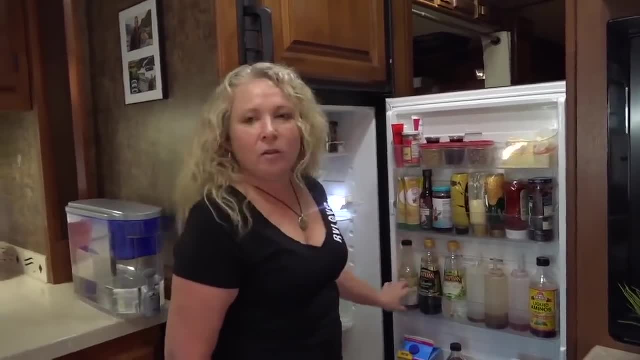 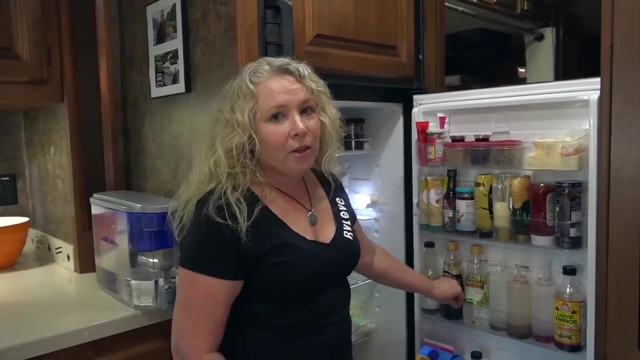 can This one's glass, but I just try not to keep too much glass in here to avoid the weight, because again, especially when you're driving, that's extra weight on the shelf and you don't want to pay $60 for it. Up here again those Rubbermaid boxes that I mentioned. 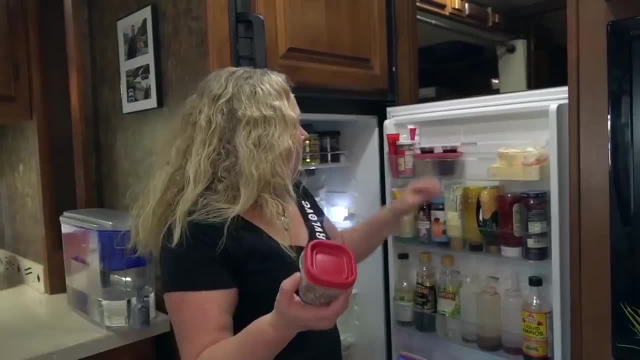 earlier, these are all plastic, So I don't want to keep too much glass in here, because these are all plastic. So I don't want to keep too much glass in here because, again, those Rubbermaid boxes are awesome for things like, you know, nuts oraries or anything. 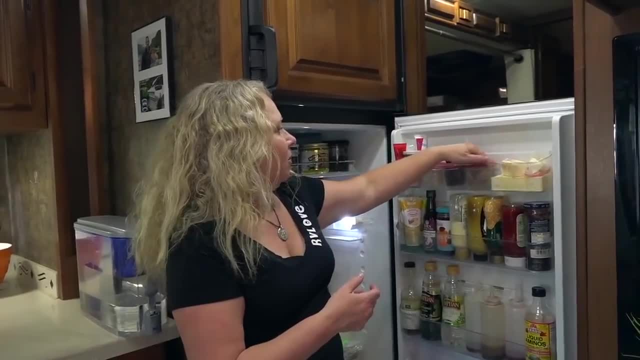 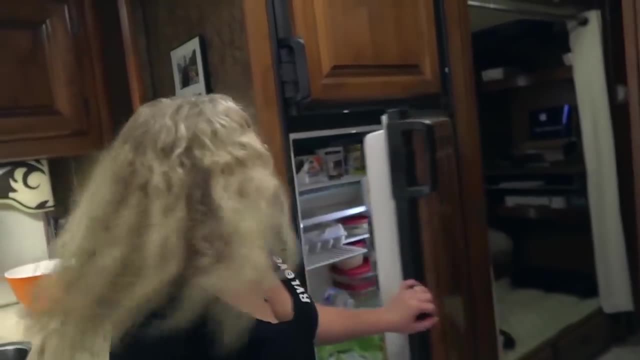 small, or if you've got small leftovers and that will fit in that top shelf really really nicely. So yeah, keep things like milk down on the bottom. That's the fridge. Let's take a look at the freezer. So RB freezers pretty small. it actually does have an ice. 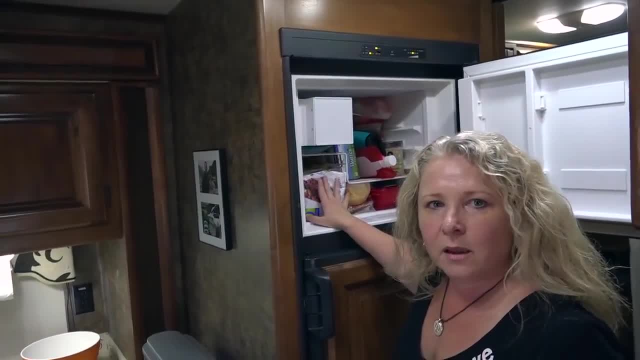 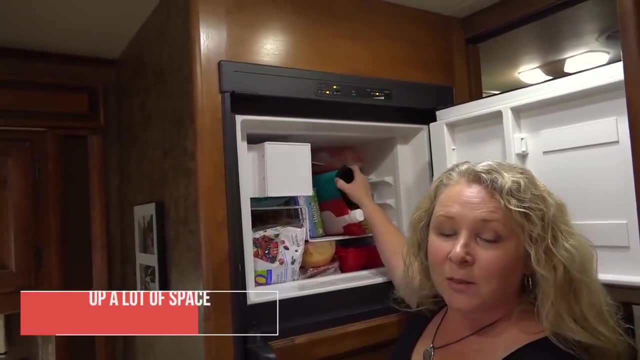 maker, but we removed the ice maker box and turned off the ice maker because we really don't use that much ice and we wanted to have the extra space for food Instead. we- and because we don't use that much ice, we make ice the old-fashioned way, using 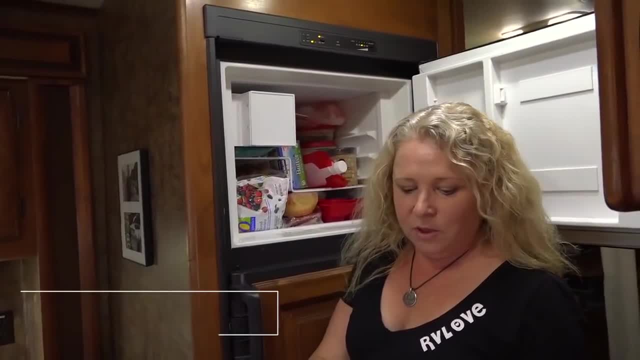 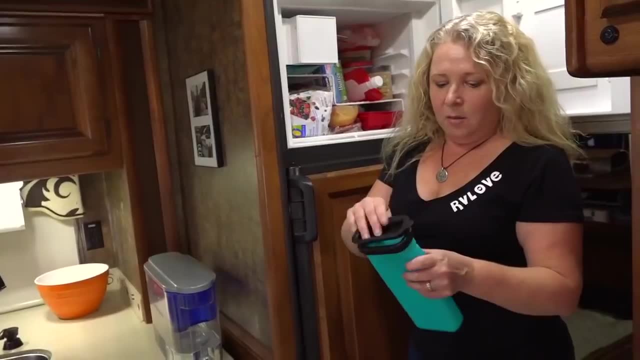 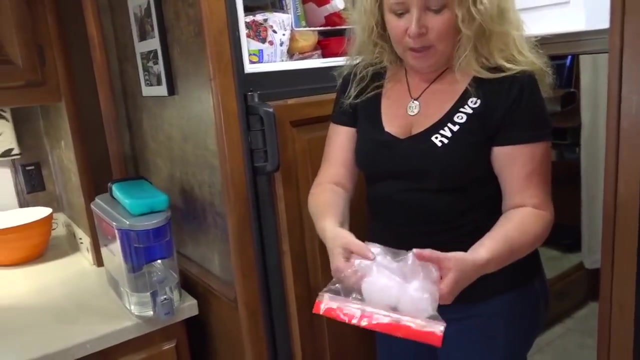 ice cube makers. this one is great because you can fill it up with water and a lid and then lay it in there and then they actually pop out as ice cubes. you could put those in a plastic bag and then keep making them big round. I feel really like ice to last you a long time. I mean these last ages, these eating it. 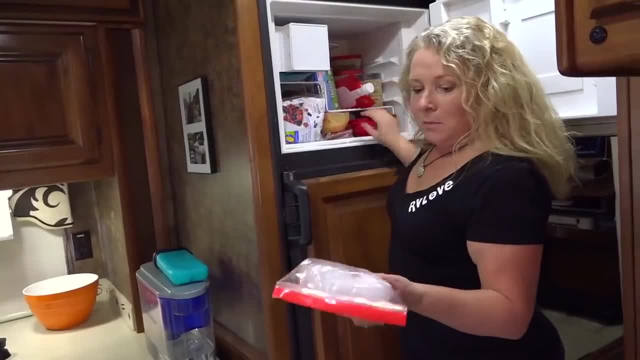 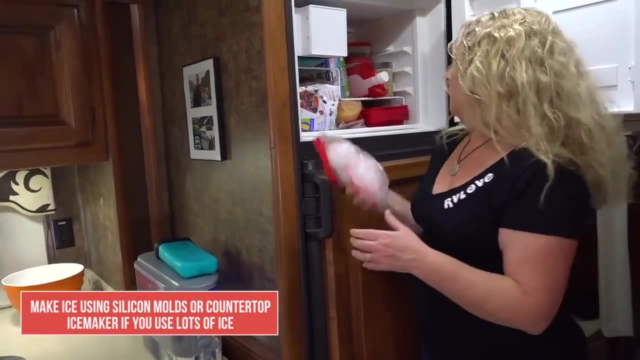 these are most liquor stores, I guess, and we got these at the makers mark when we did the distillery tour. but these huge big ice cubes will last forever and we just make them and keep them in the freezer. you can see, we don't use them very often. up here again, more of these Rubbermaid containers are super handy. 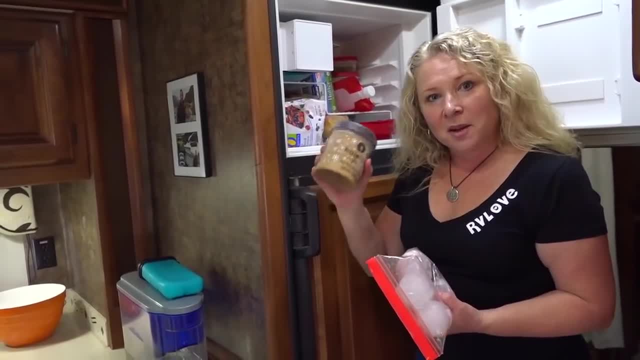 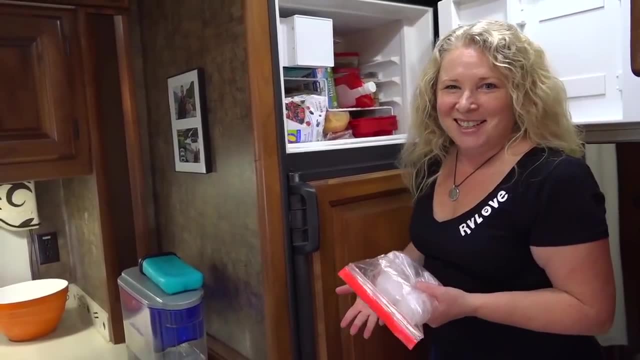 more of this Talenti sea salt caramel ice cream, which it's also handy. I don't think I need any more storage containers, but I haven't found a reason to stop buying the ice cream. this is handy. it's called wine to go, I think, so it's like a 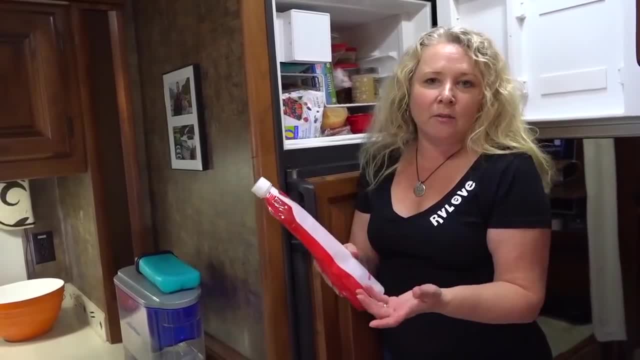 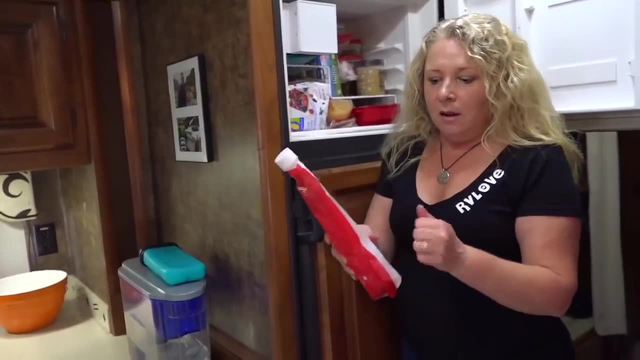 seven hundred and fifty five hundred and fifty five hundred and fifty five mil plastic flask that we fill with water. I think it's designed for wine but we fill it with water- and then we go on hikes or on a picnic. we can throw this in to keep the food cold as a ice block, but then, as it melts, we've got nice cold. 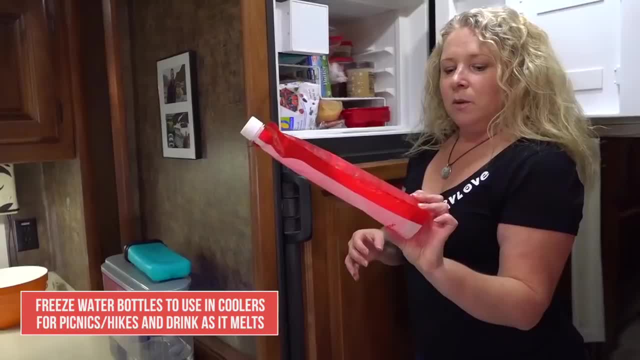 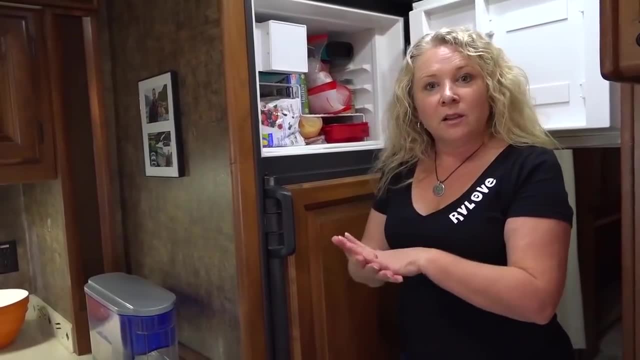 drinking water, so that is a really handy little thing as well. I'll see if I can find the link for that, and it's probably on Amazon or something, but again, containers are different shapes and sizes that lock into each other. really, really handy for your RV fridge and freezer. 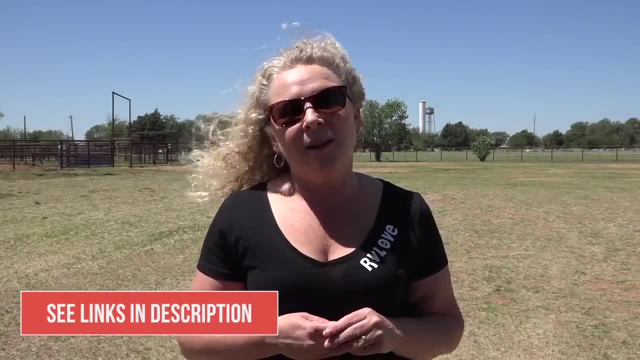 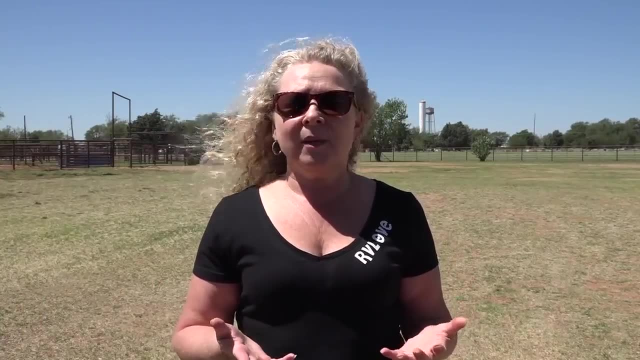 well, I hope you enjoyed today's video and got some useful tips and ideas in there. I'm curious to know what kind of fridge you have in your RV, what you like about it, what you don't, because it's just something that a lot of people are. weighing up, when they're shopping for their RV, what is going to be the best kind of RV for their needs. we've gotten by really great for four years with a, with a propane electric fridge, regular RV fridge, but we can also see huge benefits to having a residential. so we'd love to hear your thoughts and ideas pop.